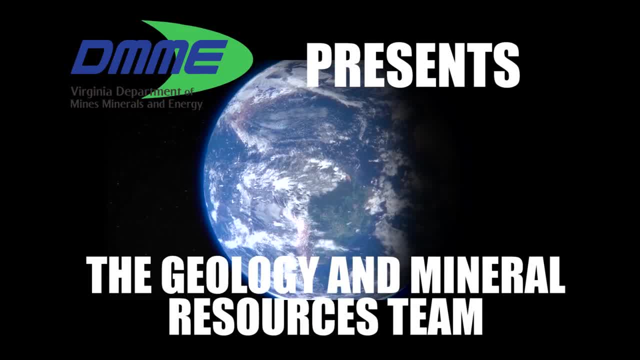 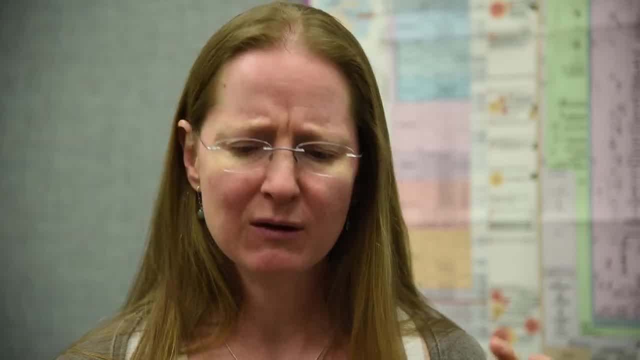 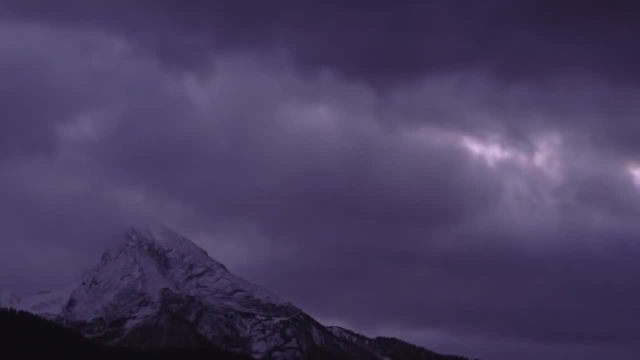 It's so big. It's huge. I mean it's the study of the earth and how it functions and works and how everything links together. So it's basically just a holistic understanding of the earth- Geology. It is the foundation of nearly all the work done at the Virginia Department of Mines, Minerals and Energy. 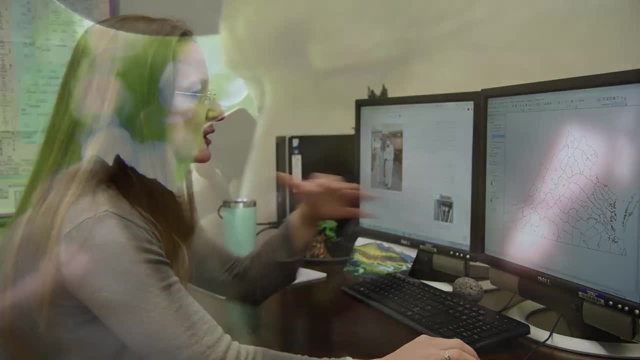 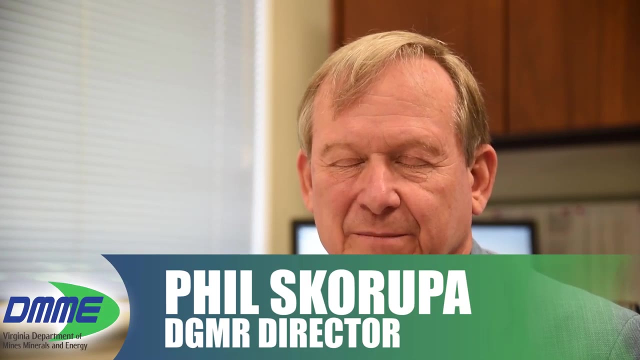 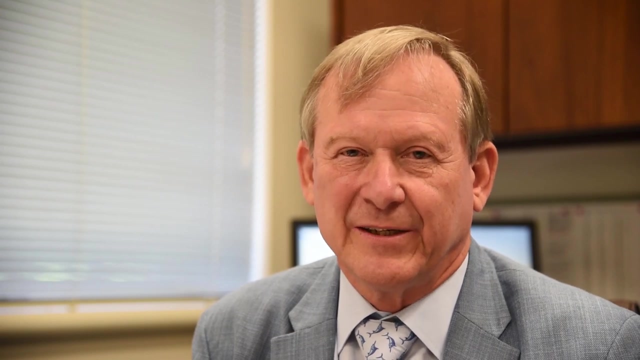 The geology team is made up of 11 scientists and includes Virginia's state geologists. They hold a lot of value because they are the record keeper. They have all the mineral resources, the records for that They are the repository, for that They maintain the records and do a lot of mapping in the state of Virginia. 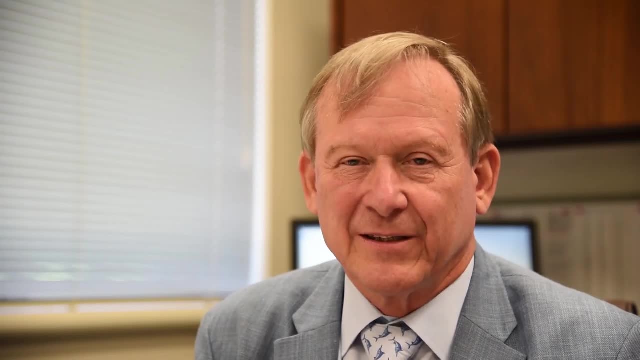 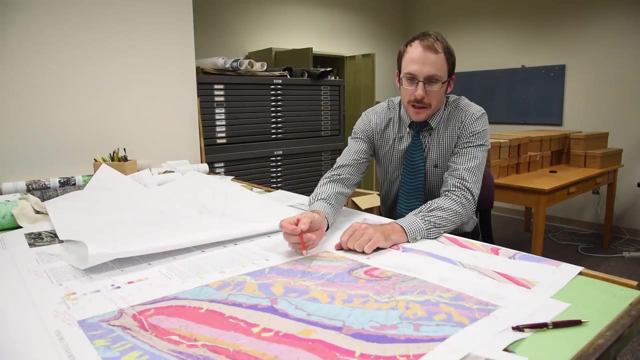 And a lot of valuable things that contribute to both the economy and contribute to the mining industry. The geology team is divided into two sections: economic geology and mapping. Our main product in those projects are geologic maps that are used by a variety of people. 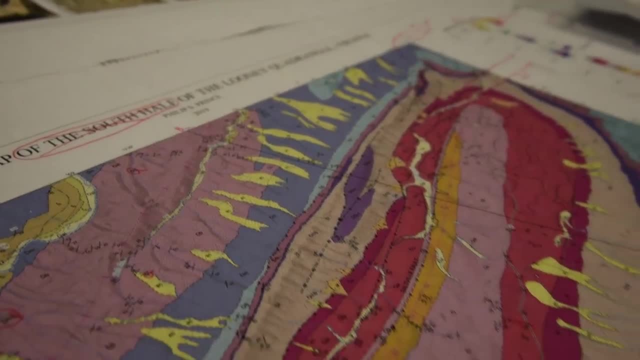 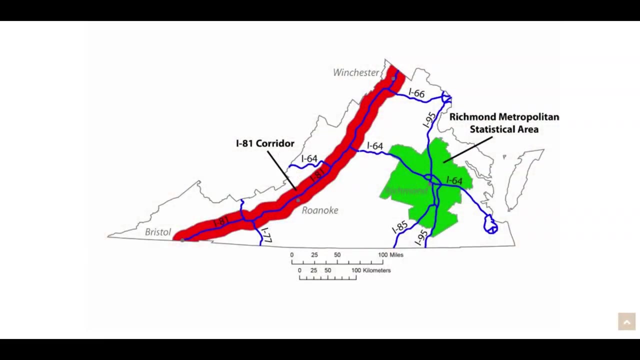 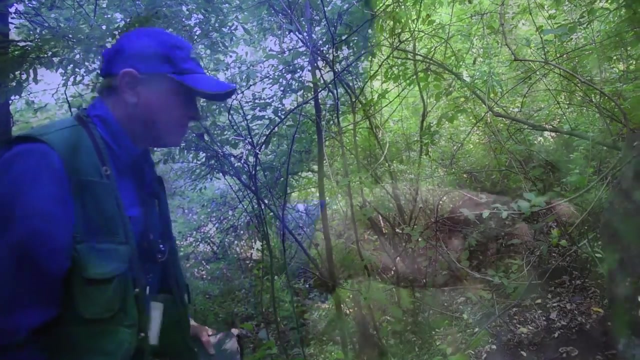 Funded by a grant from the US Geological Survey, DMME geologists are currently mapping areas where development is happening: The I-81 corridor and the Richmond metro area. They start in the field, observing outcrops and other land features. 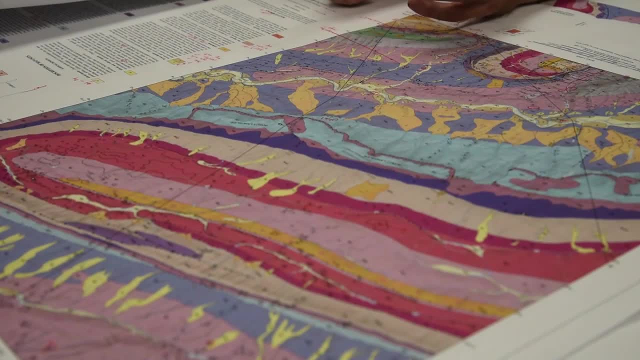 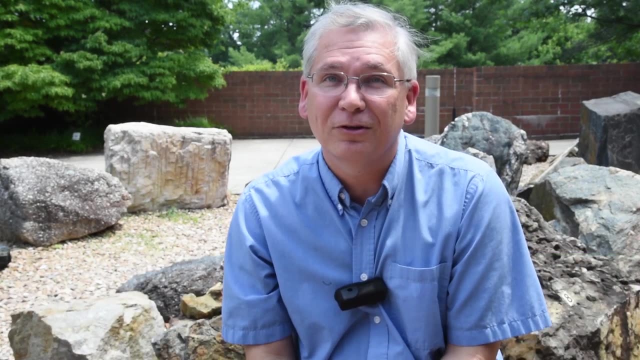 They also use photos and LIDAR images to come up with the final product. I often tell people that geologic maps are like a forecast for the earth. Once you start to do something To develop that land, You really do want to have an understanding of what's under the ground. 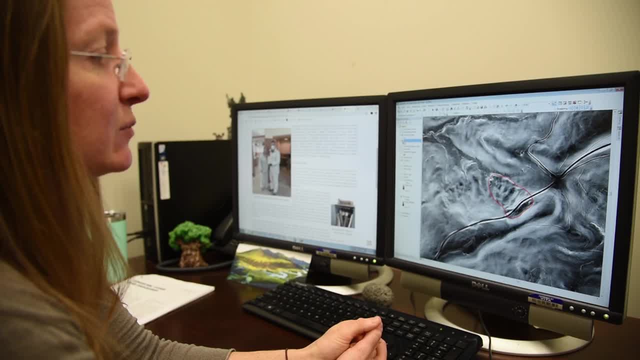 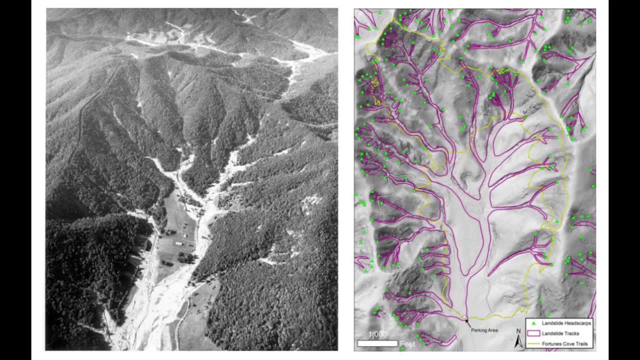 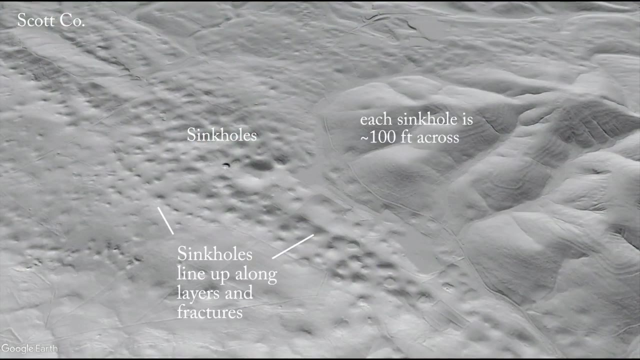 The geology team maps geologic hazards. A federal emergency management agency grant has the scientists looking for historic, current and the potential for landslides in Nelson and Albemarle counties. They also track karst and sinkholes, as well as fault lines to better notify those at potential risk for earthquakes. 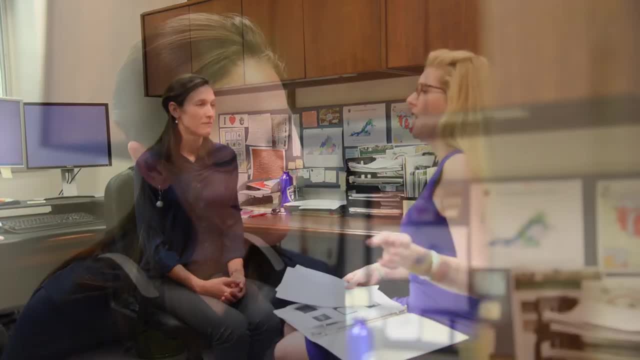 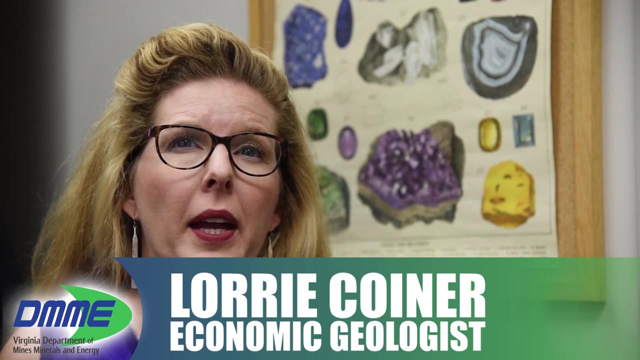 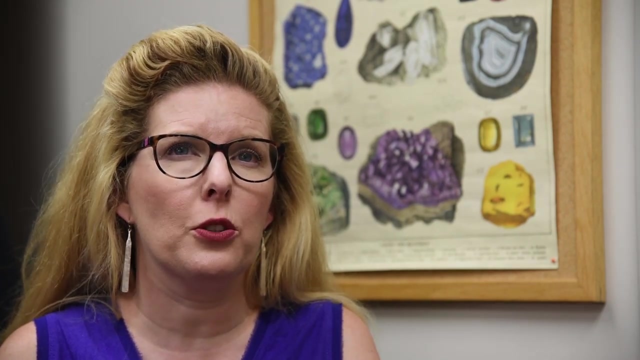 That information is available on our website. That information is available to anyone And, as part of the economic geology program, is being shared with localities. We try to make sure that the people who make land use plans for local communities have all the information they need to make wise land use decisions.